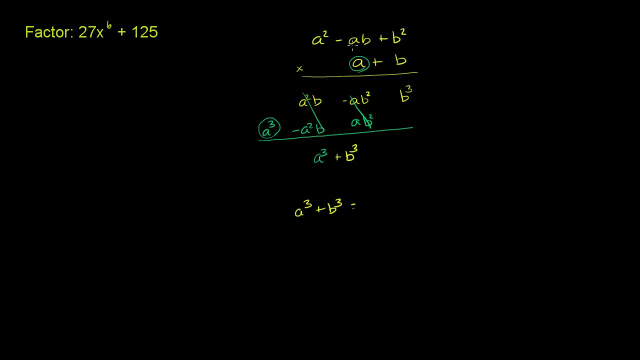 a to the third plus b to the third. this can be factored into these two expressions. That can be factored into a plus b times a squared minus ab plus b squared. So this is essentially the special form. If you have a sum of cubes, it can be factored out. 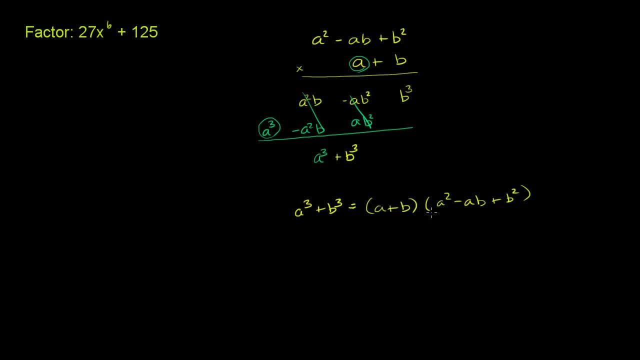 as the sum of these, The sum of the cube. roots times this expression right here And we just showed that it works. So let's see if we have that special form here. Well, 27 is definitely the cube of 3.. 3 to the third power is 27.. 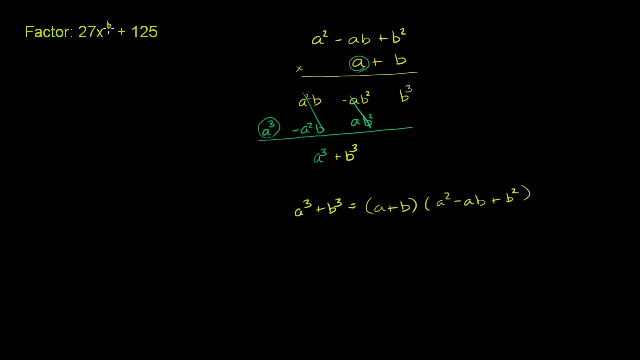 x to the sixth is also the cube of x squared. If you raise x to the sixth to the 1 third power, you get x squared. So this first term right over here can be rewritten as 3x squared to the third, And the second term right here, that's 5 to the third power. 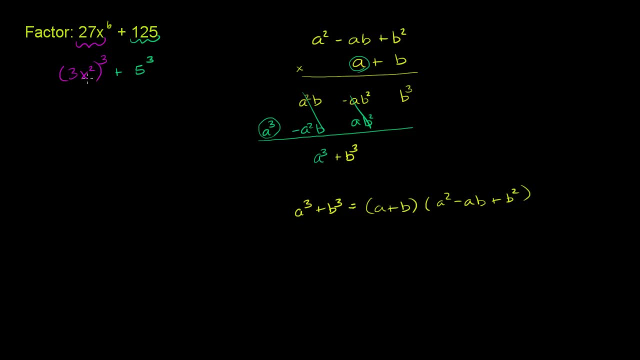 So plus 5 to the third power, And this might be a little bit confusing for you, So it never hurts to review. Let's multiply: 3x squared times 3x squared times 3x squared, That is literally equal to 3 times 3 times 3 times x squared. 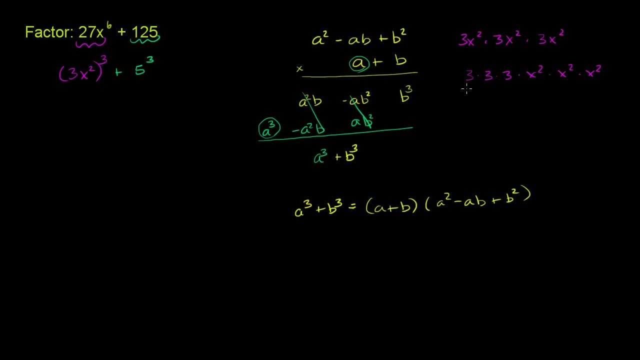 times x squared. times x squared: This part right here is 27.. x squared times x squared is x to the fourth. It's times x squared is x to the sixth, Or you could just raise both of these to the third. power 3 to the third is 27.. 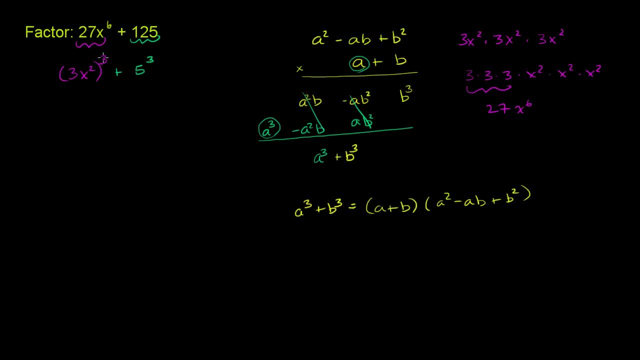 x squared to the third power. You take an exponent to an exponent And you're going to take the product of the exponent, So it'll be x to the 2 times 3, or x to the sixth power. So now we know that we have this pattern. 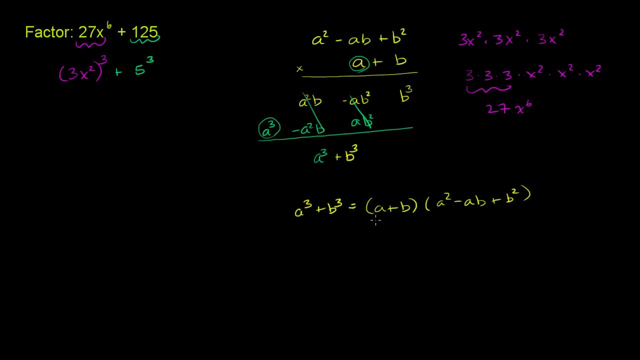 So we can just use this. We have the sum of cubes, So just by using this pattern right over here, that means that we can factor it, as this is going to be equal to 3x squared. That's our a. Let me make it clear. 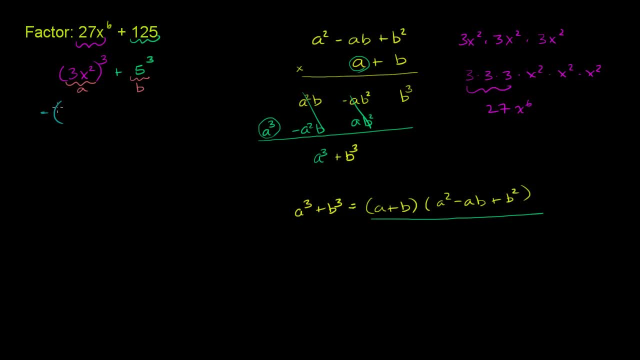 This right here is our a. This right here is our b. So it's going to be a plus b, So it's going to be 3x squared plus b plus 5 times a squared. Let me do this in a new color.